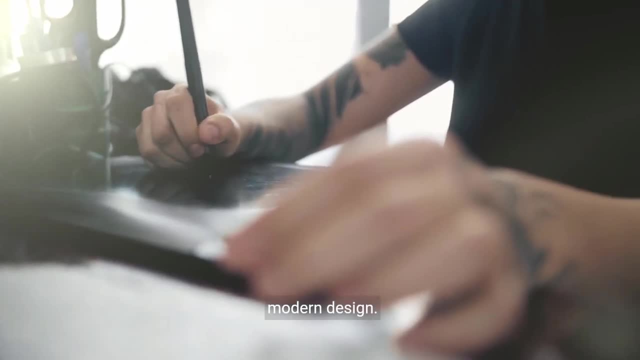 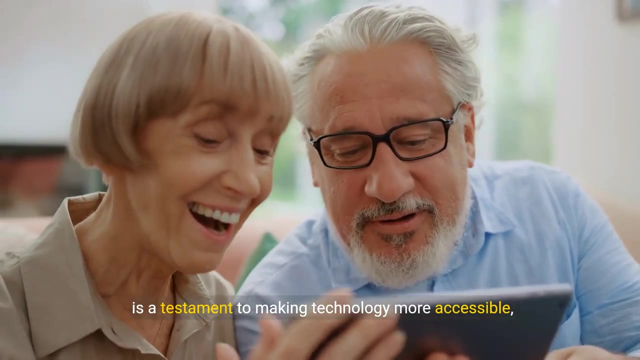 This is not science fiction, but the aim of HCI in modern design. The journey of HCI, spanning decades since computing's dawn, is a testament to making technology more accessible, efficient and enjoyable. This historical backdrop is not just context but the cornerstone. 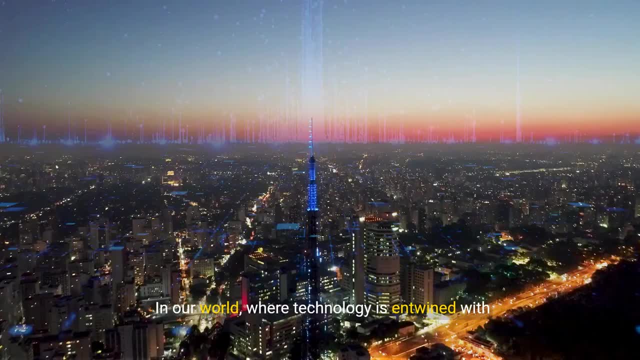 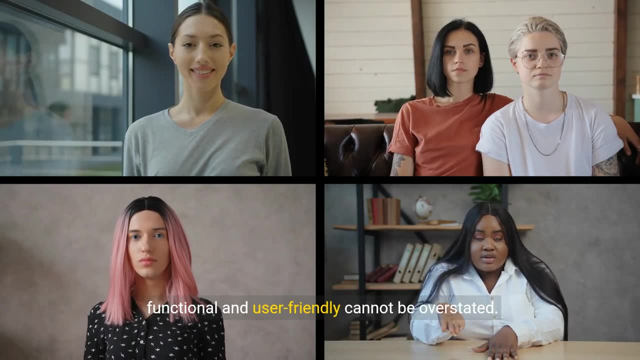 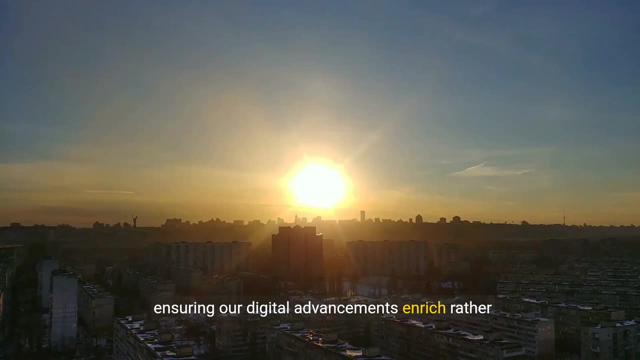 in forming today's user interface innovations. In our world, where technology is entwined with daily life, the significance of designing interfaces that are functional and user-friendly cannot be overstated. HCI stands at the intersection of technology and humanity, ensuring our digital advancement. 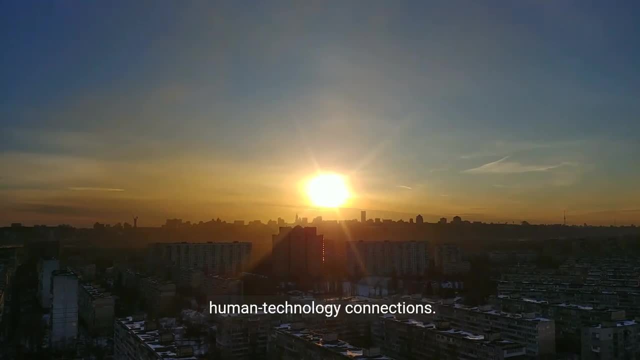 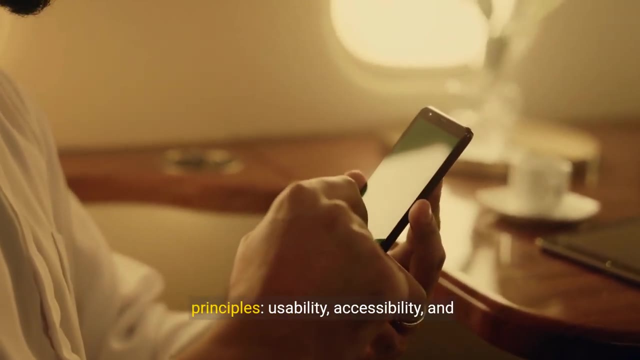 enrich rather than complicate, promising more meaningful human technology connections. Delving further into HCI, we encounter its core principles: usability, accessibility and ergonomics. Far from mere buzzwords, these are the pillars that ensure technology fulfills its purpose. 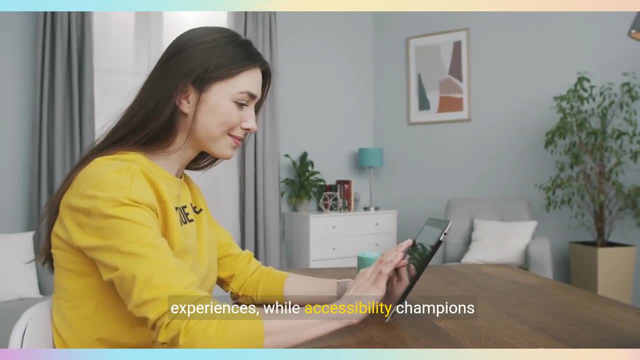 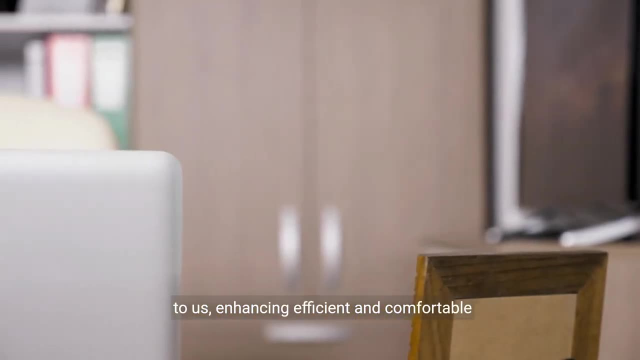 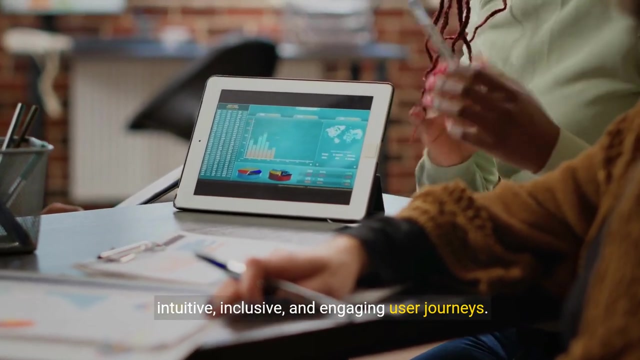 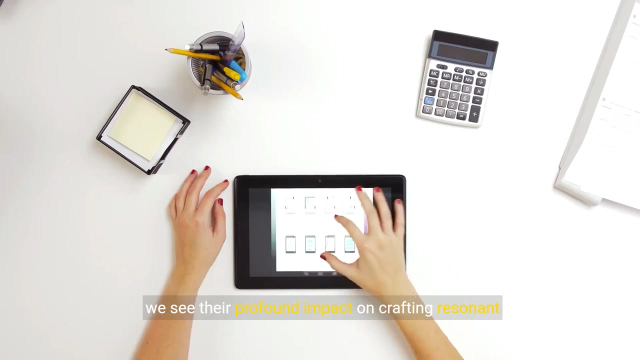 Usability transforms interactions into joyous experiences. while accessibility champions inclusivity, Ergonomics emphasizes that technology should adapt to us, enhancing efficient and comfortable interactions. These principles are instrumental in designing intuitive, inclusive and engaging user journeys. As we explore how these principles inform user interface strategies, we see their profound 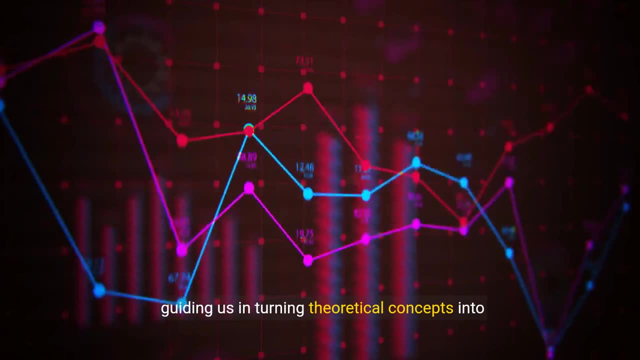 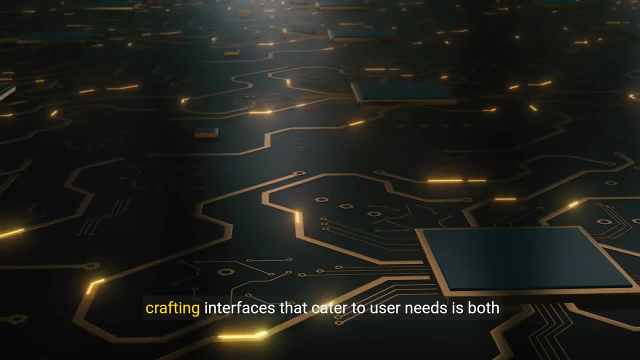 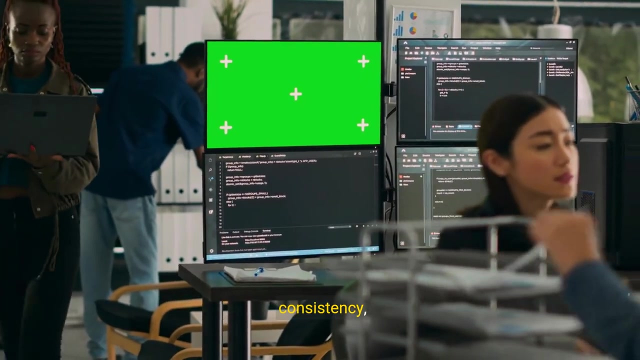 impact on crafting resonant experiences, guiding us in turning theoretical concepts into practical applications. In the nuanced world of user interface design, crafting interfaces that cater to user needs is both an art and a strategy. Central to this endeavor is the principle of consistency, ensuring users navigate digital realms with ease. In addition, responsive design. 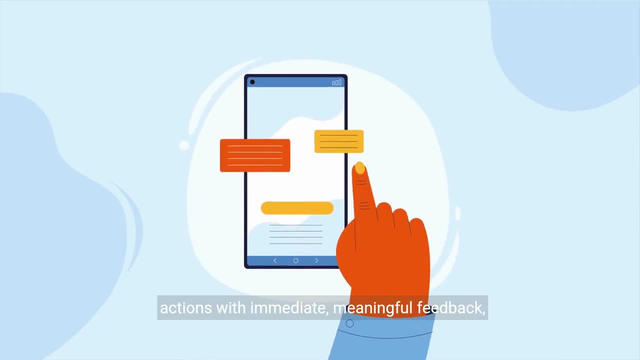 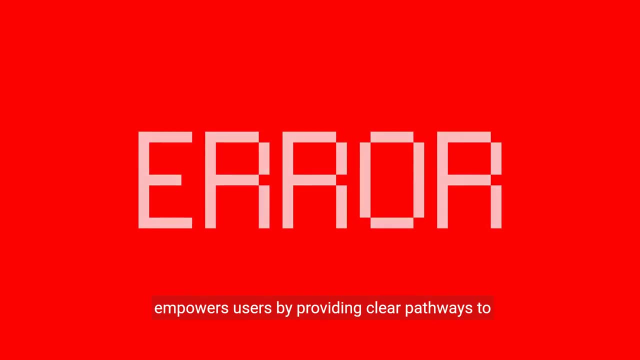 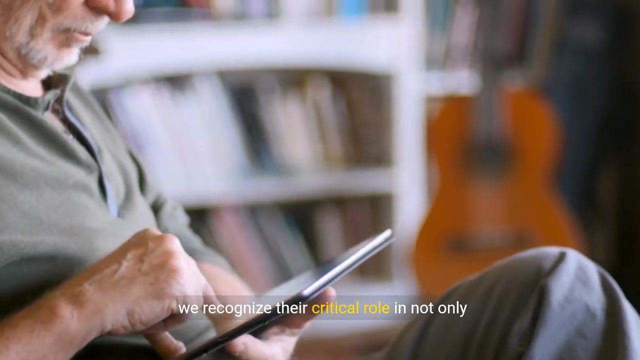 acknowledges user actions with immediate, meaningful feedback, enhancing engagement. Importantly, designing for error recovery. empowers users by providing clear pathways to correct mistakes, fostering resilience. As we explore these strategic principles further, we recognize their critical role in not only advancing user experience, but also in emphasizing the transformative 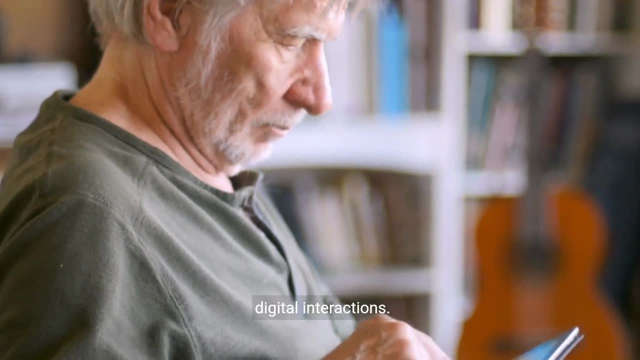 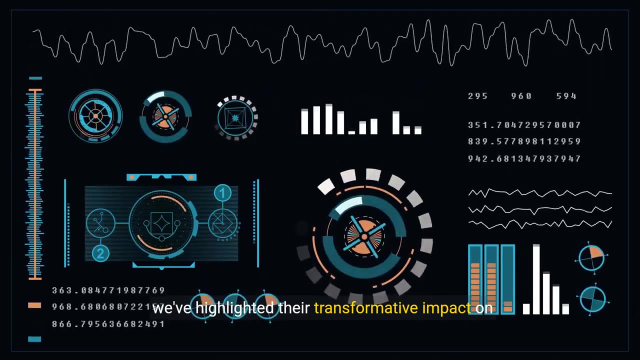 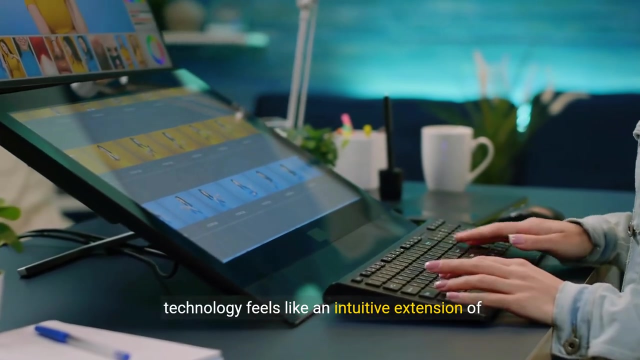 power of HCI. Through our exploration of HCI principles and user interface strategies, we've highlighted their transformative impact on user experience. HCI enhances usability to such an extent that technology feels like an intuitive extension of ourselves, elevating user satisfaction and forging a positive, engaging relationship.